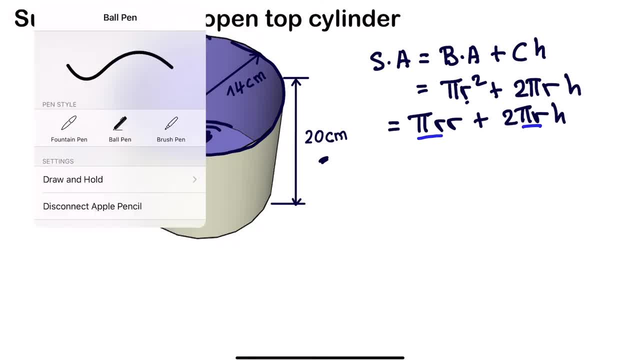 side. so factorization will help us to calculate easily without making mistake. so this is the same. as we are going to have PI R bracket, so will be left here. so we have R. here we are left with 2 Rh, so we have 2. we have 2s, so here we're left with 2h, so we 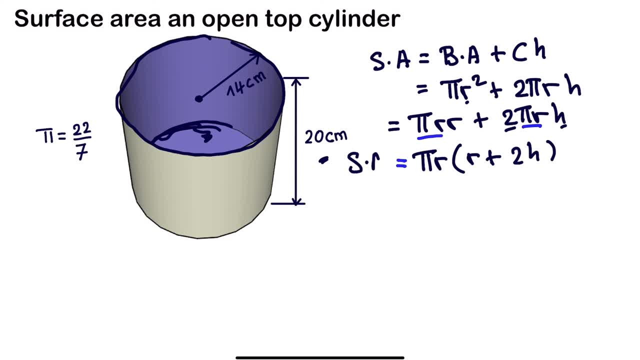 have to each. so this is our formula for surface area of an open top cylinder. so we can use this formula and substitute the values. so our surface area will be equals to PI. PI is 22 over 7, 22 over 7 times the radius. this is our radius R. 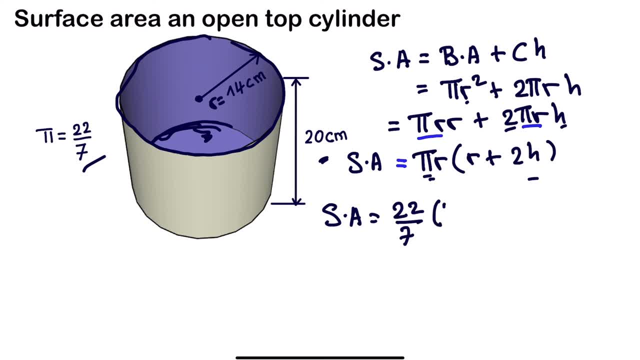 is 14 bracket. we have R again, which have 14 plus 2 H. 2 H is 20, 20. so if we want to simplify this, we are going to have: for 7 divided by 14 is 2, so we are going to have 22 times 2, and if we add this, if we 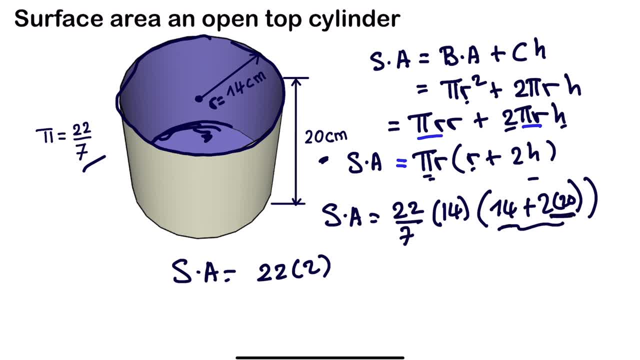 multiply this, we have 40 plus 14. so we are going to have another bracket. 14 plus this is 2 times 20 is 40. this will give us 44 bracket. if we add this together, we have 54. so 54 times 44. 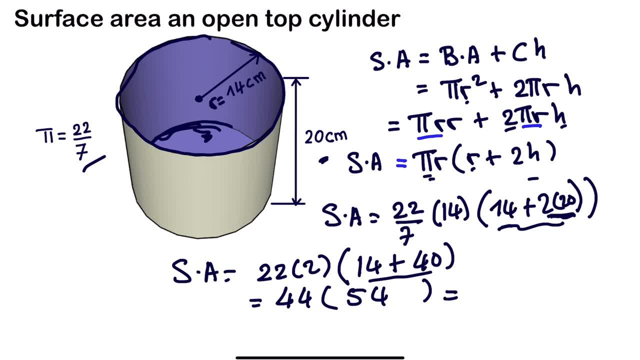 this will be equals to 2376 centimeter square, so this is our surface area. so thanks for watching. please subscribe.